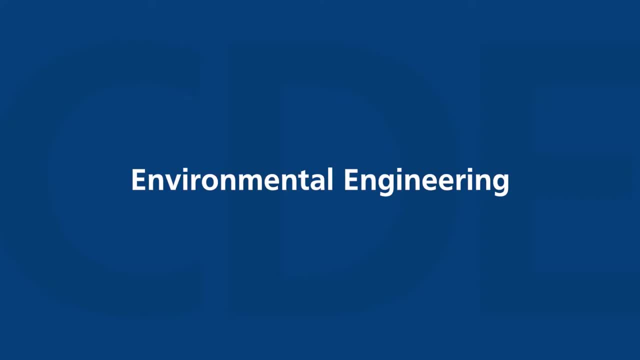 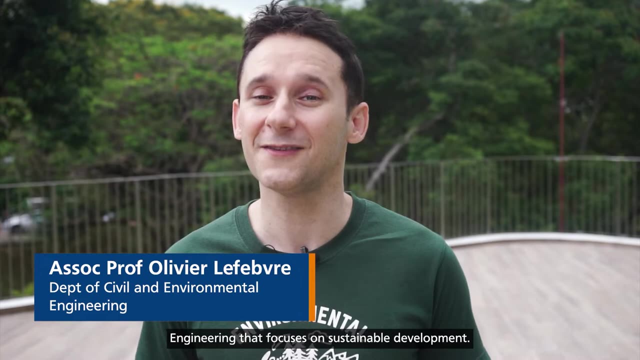 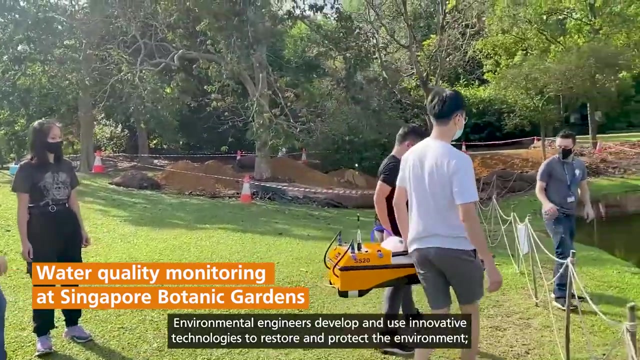 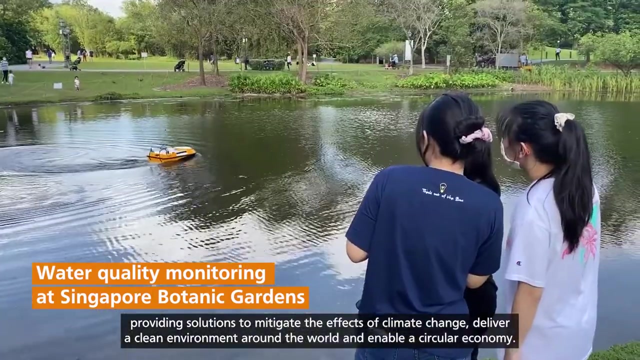 Environmental engineering is a fast-growing branch of engineering that focuses on sustainable development. Environmental engineers develop and use innovative technologies to restore and protect the environment, providing solutions to mitigate the effects of climate change, deliver a clean environment around the world and enable a circular economy. 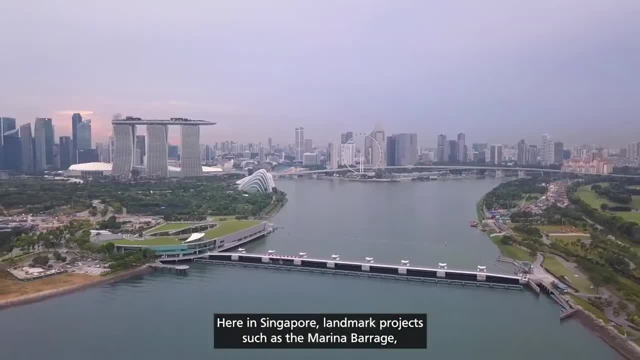 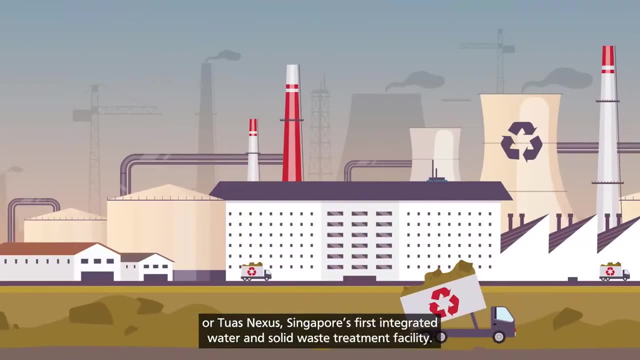 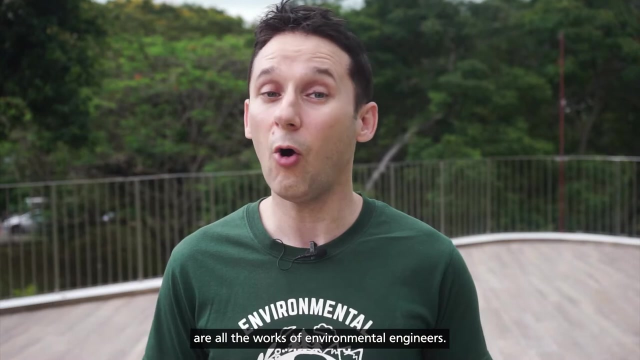 Here in Singapore, landmark projects such as the Marina Barrage, the New Water Purification Plants, the Lorong, Halus Wetland or Tuas Nexus, Singapore's first integrated water and solid waste treatment facility, are all the works of environmental engineers. 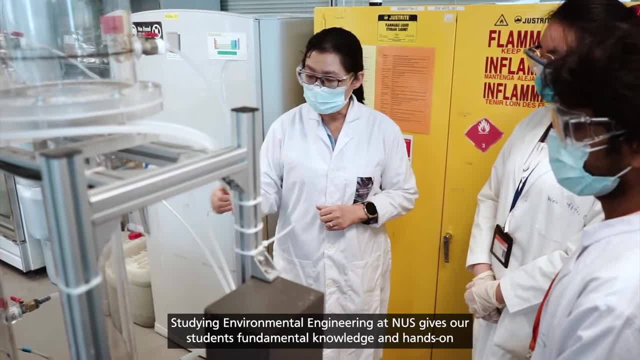 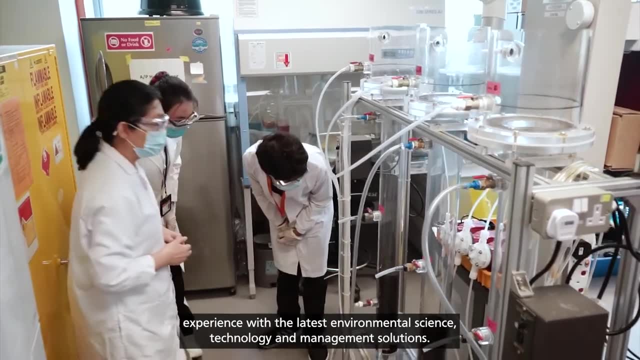 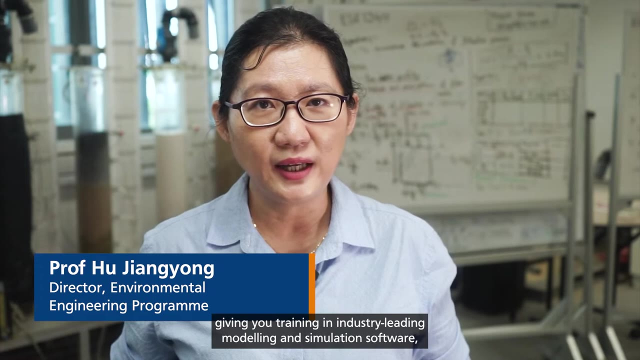 Studying environmental engineering at NUS gives our students fundamental knowledge and hands-on experience with the latest environmental science technology and management solutions. At NUS, we are at the forefront of digitalization, giving you training in industry-leading modeling and simulation software, as well as exposure to 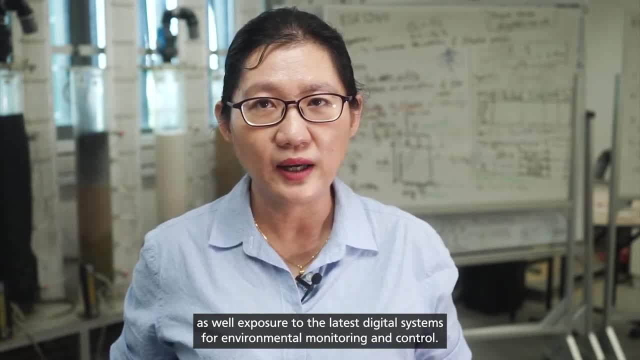 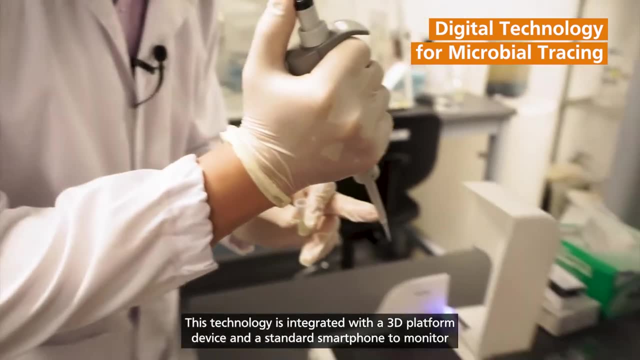 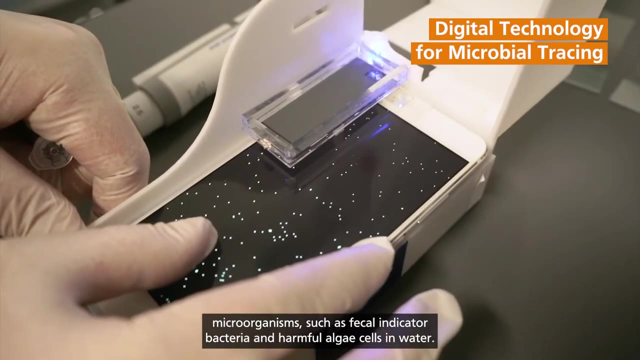 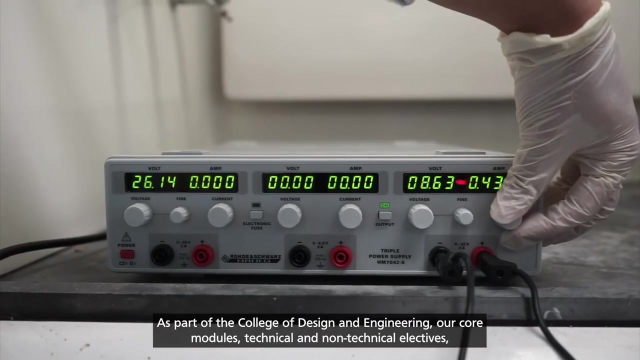 the latest digital systems for environmental monitoring and control. This technology is integrated with a 3D platform device and standard smartphone to monitor microorganisms such as microorganisms in water. As part of the College of Design and Engineering, our core modules- technical and non-technical electives- capstone design project. 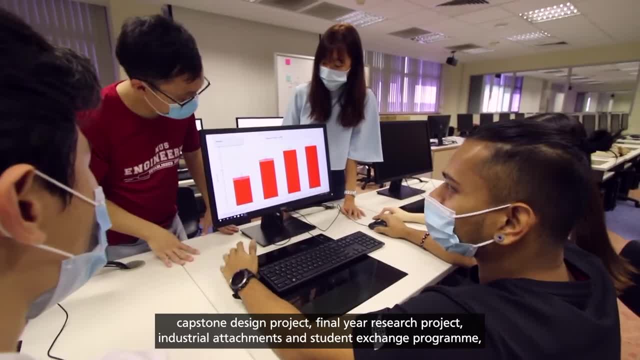 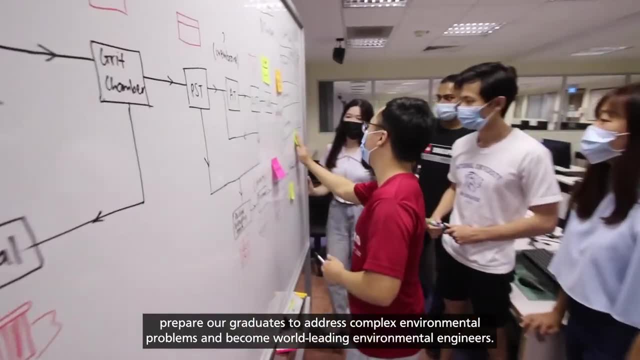 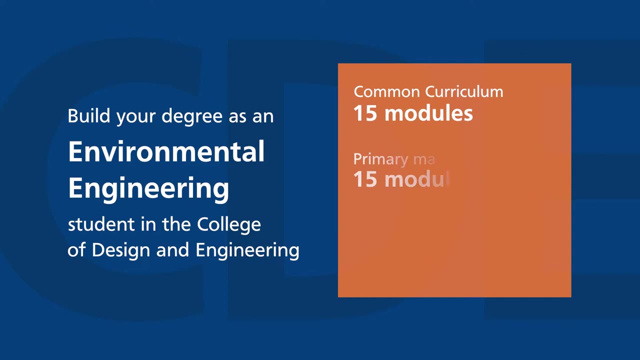 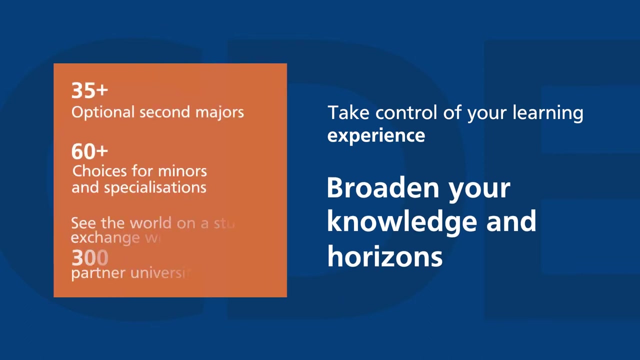 final year research project, industry attachment and student exchange program prepare our graduates to address complex environmental problems and become world-leading environmental engineers. While student life is very fulfilling here, our events are run by the Environmental Science and Engineering Students Club, in short EZ, a club that represents the environmental engineering student. 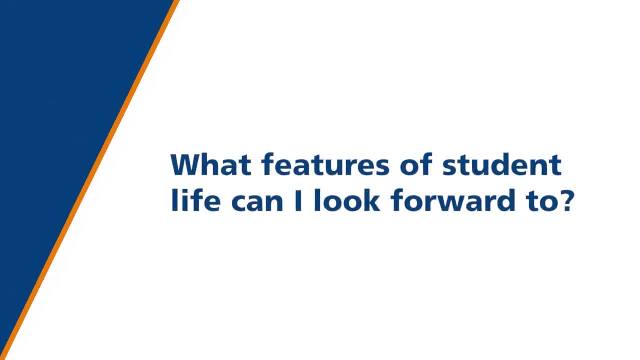 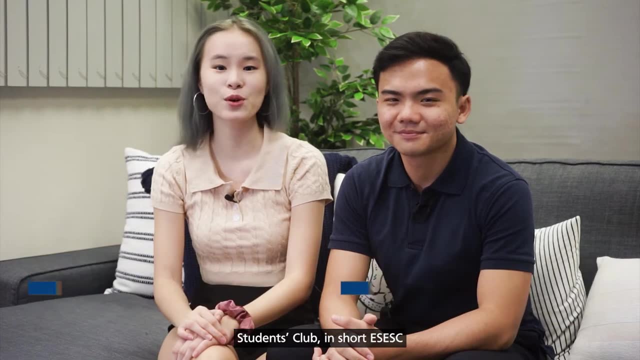 body. We aim to instil a sense of belonging in the environmental engineering community, where every student matters. EZ's club will be a place where you can connect with one another and share your thoughts, thoughts and ideas. We also invite students to move along and share their experiences. 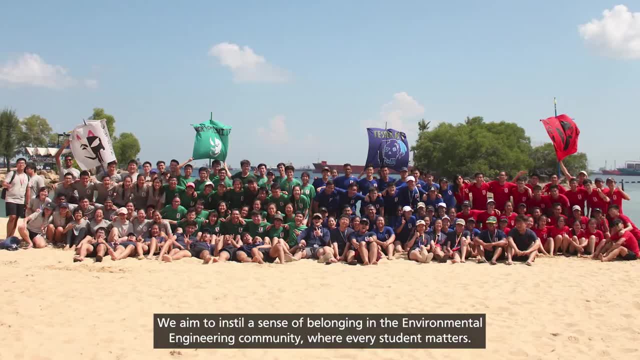 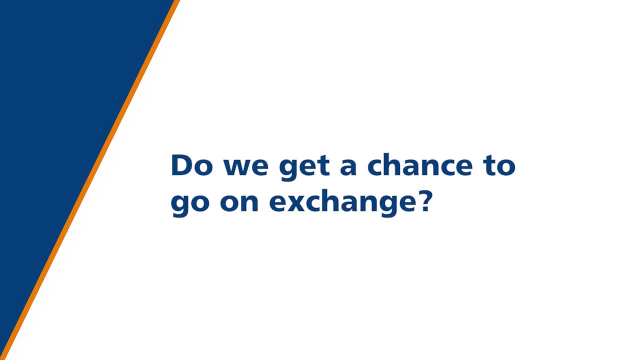 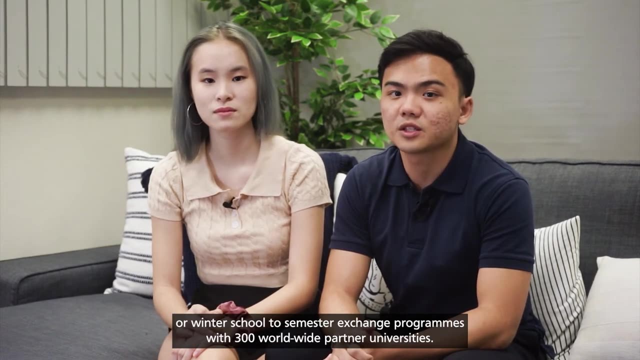 with each other. For example, we have a conference where we can exchange ideas and ideas about environmental science and engineering. We also have an event where we can meet students. The flexible curriculum at NUS means students can get at least one overseas exchange experience from summer or winter school to semester exchange programmes with 300 worldwide partner universities. 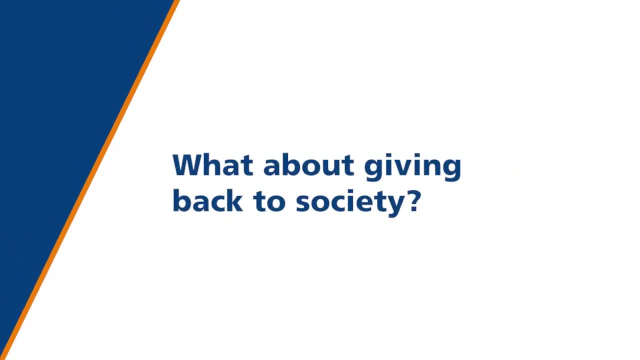 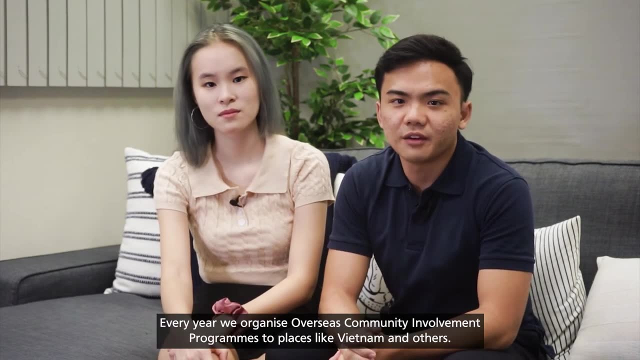 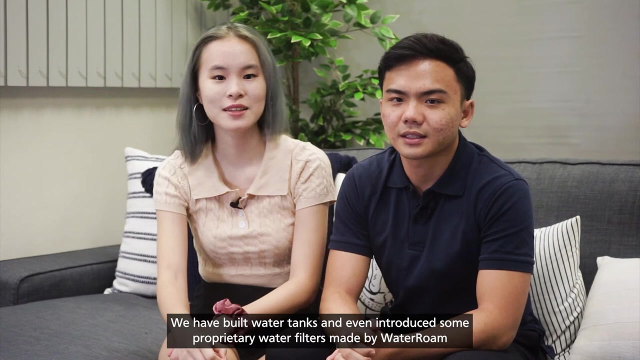 More importantly, it is grade-free. As environmental engineering students, we believe in building a better world for tomorrow. Every year, we organise overseas community involvement programmes to places like Vietnam and others. We have built water tanks and even introduced some proprietary water filters made by WaterRoam. 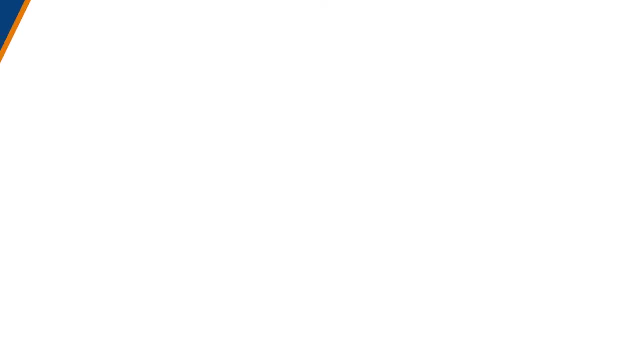 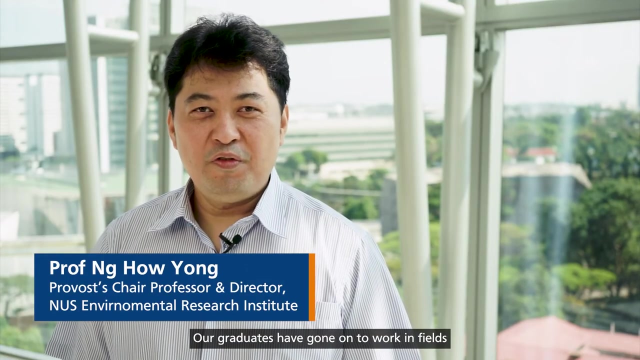 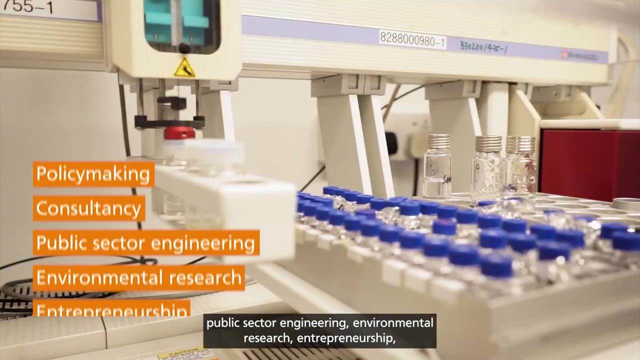 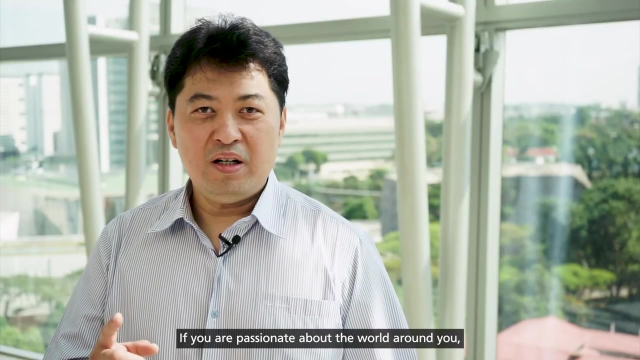 a start-up run by environmental engineering alumni. Our graduates have gone on to work in fields such as policy-making, consultancy, public sector engineering, environmental research, entrepreneurship and healthcare. If you are passionate about the world around you, studying environmental engineering opens. 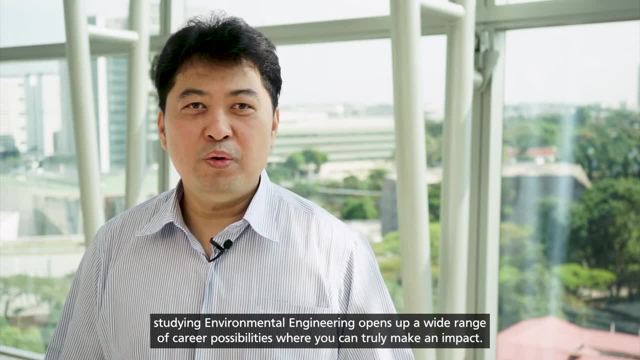 up a wide range of career possibilities where you can truly make an impact. 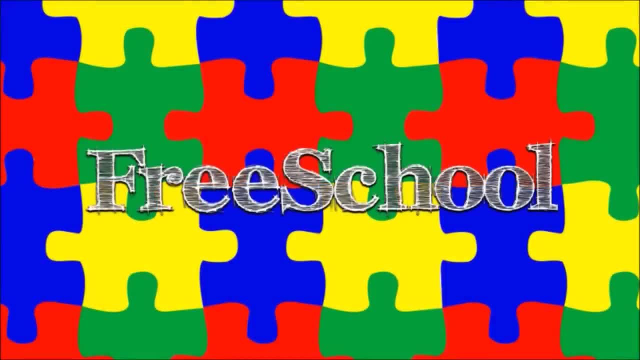 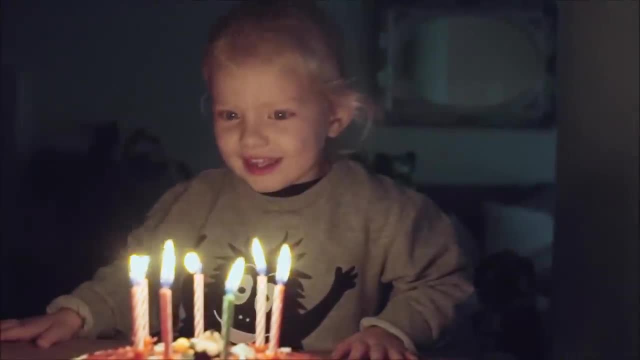 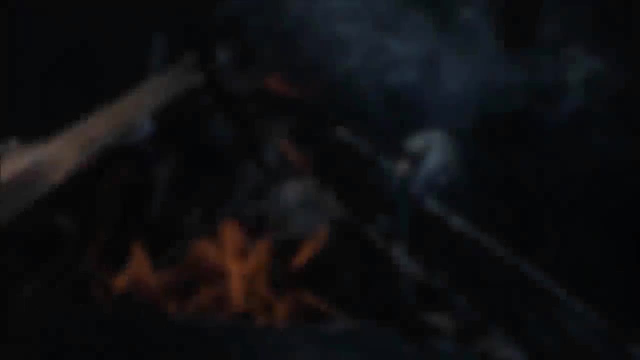 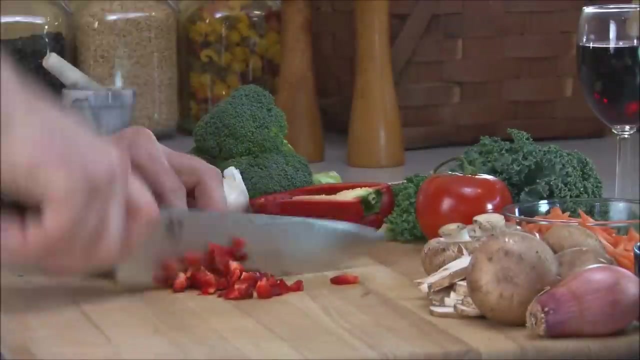 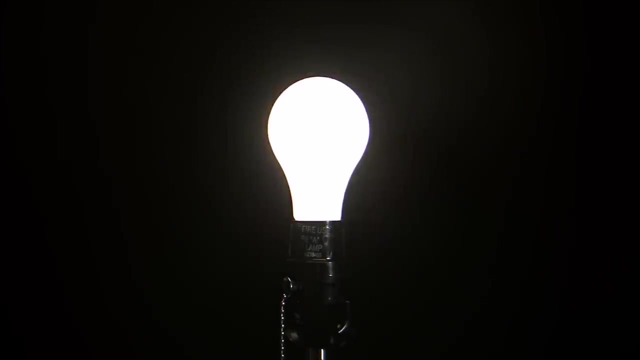 No matter where you are or what you are doing, things are changing all around you. Whether it's plants growing or logs burning, or even if you're just eating food, the materials around you are changing in size, shape and structure, releasing or absorbing energy, and 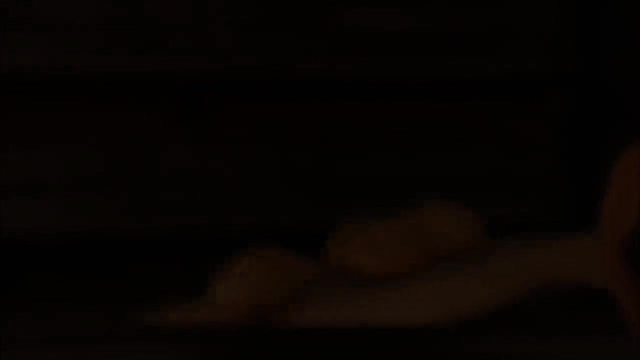 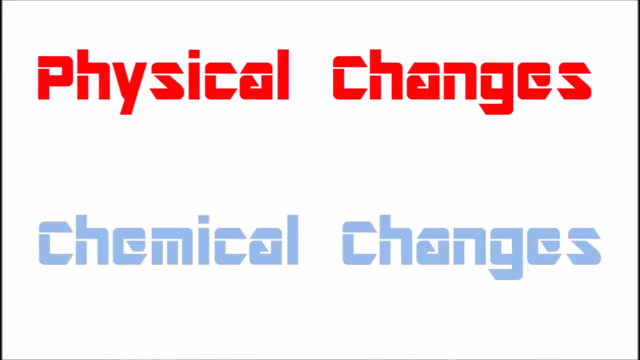 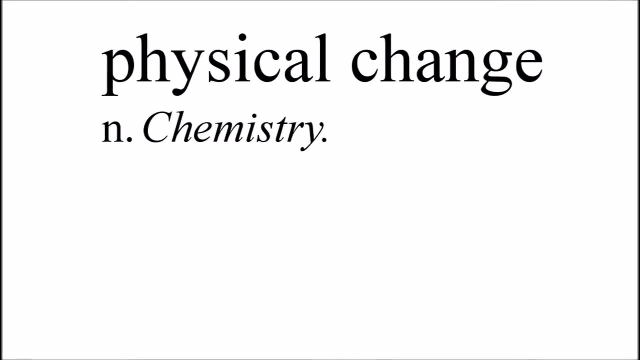 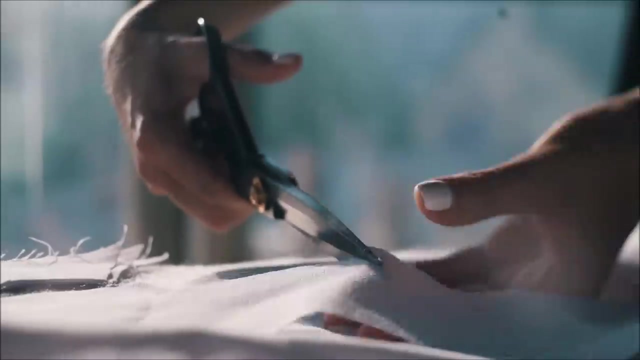 creating new substances. In chemistry, most changes are divided into two categories: physical changes and chemical changes. A physical change is something that changes the physical properties of an object or substance, like size, shape or form. Cutting a piece of cloth is an example.